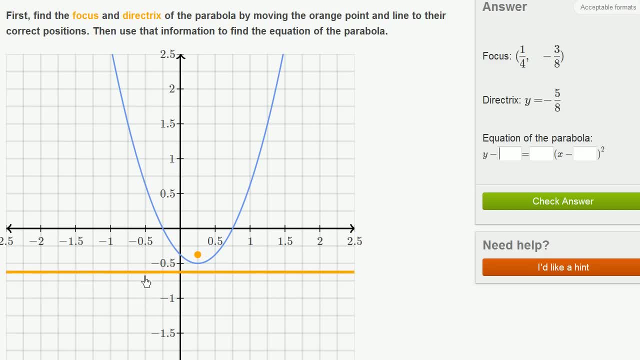 my directrix up there. that should work out, So let me move it up there. And there you have it. Notice now my parabola. these green lines show the distance to the focus and the distance to the directrix, And notice that they are always the same. 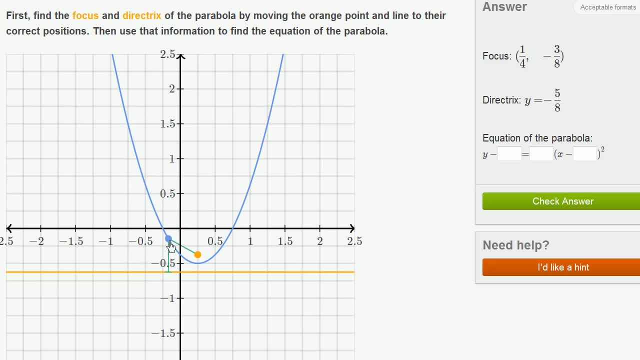 So it looks like I got the right focus and the right directrix now. So I got the right focus and the right directrix. And the focus is one-fourth comma, negative three-eighths, and the directrix is: y equals negative five-eighths. 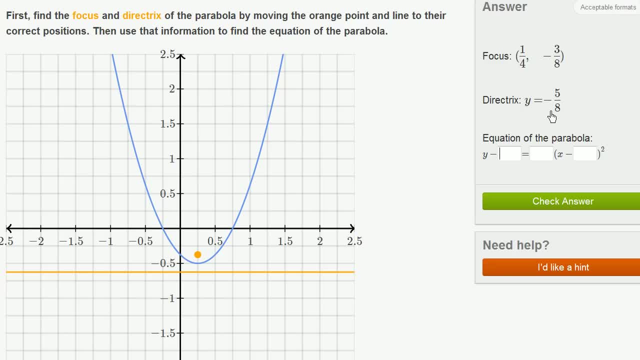 So now let's try to use that information to actually find the equation of the parabola in this form right over here, And this is going to involve a little bit of algebra for us, So let me copy and paste this so that we know what we need, And let me open my little scratch. 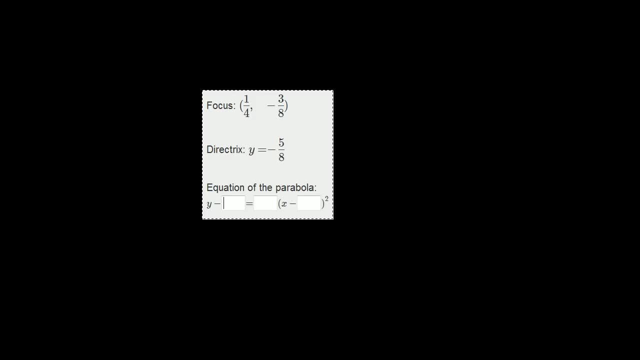 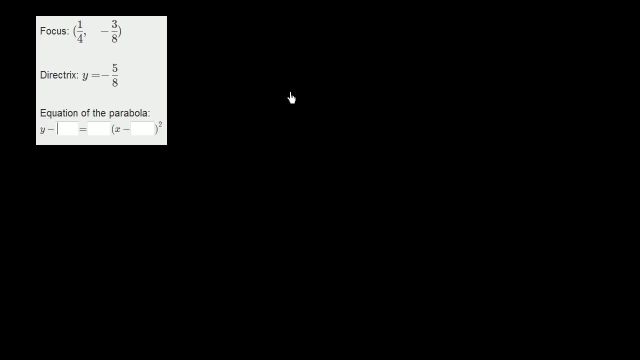 pad up. So this is our information And we need to figure out the equation of the parabola. So, just as a little bit of review, we have the point. So let's say this is our point, This is our focus. It's the point one-fourth comma, negative three-eighths. And then we 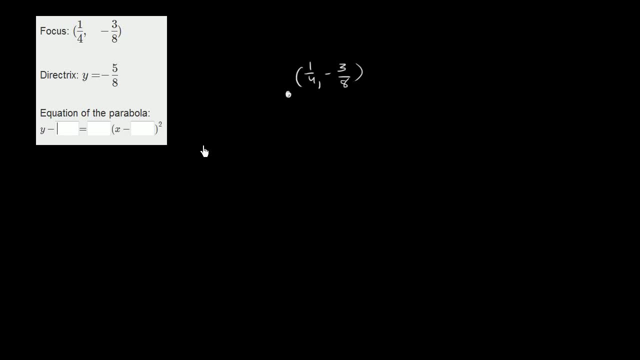 have the directrix. So the directrix looks something like this. The directrix looks something like that: That is, y is equal to negative five-eighths, And then we have our parabola. We have our parabola and it looks something like this: 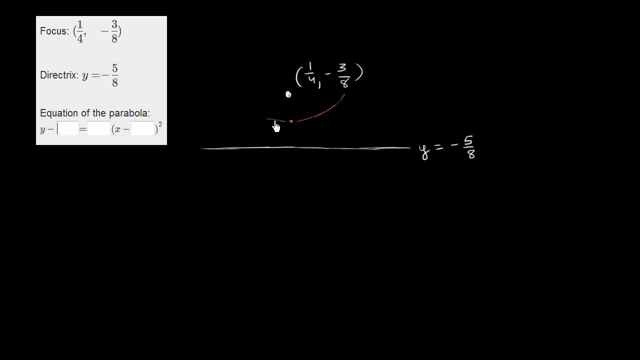 It's equidistant to the two. So our parabola looks something like that And the parabola, the x's and y's that satisfy this equation are all of the x's and y's that are equidistant to these two things. 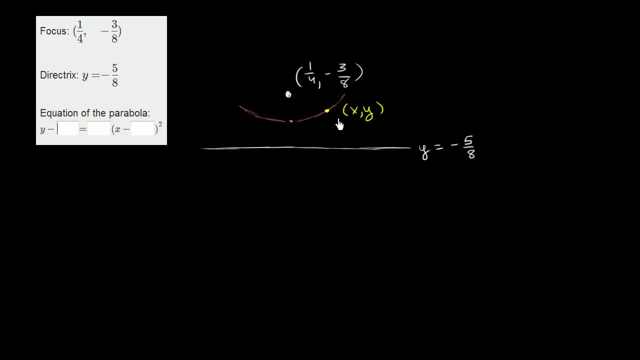 So let's call that y. So let's find an equation for all of the x's and y's that are equidistant to this point and to this line right over here. So first let's think about the distance between this focus and this xy right over here. 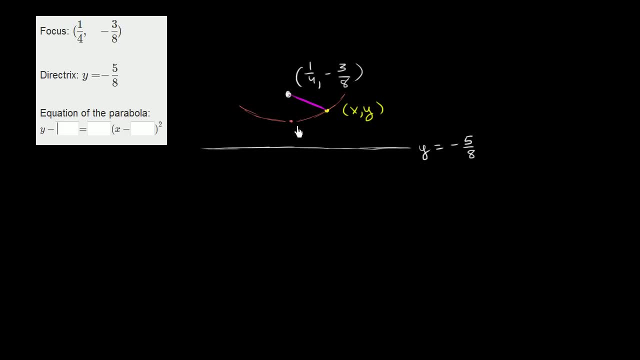 Well, that distance just comes straight out of the distance formula, which comes straight out of the Pythagorean theorem. It's going to be x minus one-fourth squared, plus y minus minus negative 3 eighths squared. So that's going to be y plus 3 eighths squared. 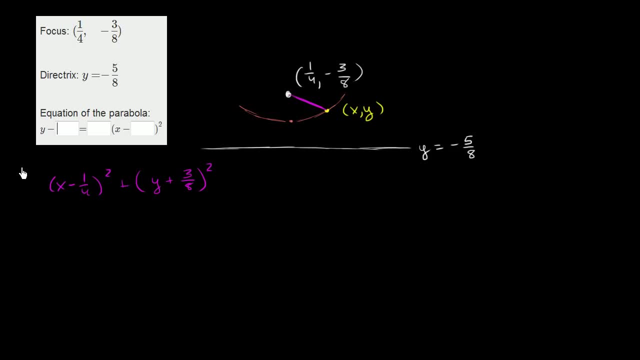 So this is our distance squared. We could take the square root if we. let me just do that. So let me just take the square root. So this is the distance between any point on the parabola xy and the focus, And the distance between that same point and the directrix. 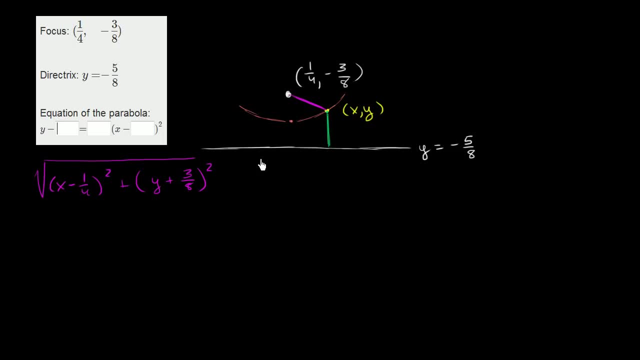 well, that's just going to be a straight vertical line. So that's just going to be our change in y. So this is going to be equal to y minus negative 5 eighths, which is the same thing as y plus 5 eighths. 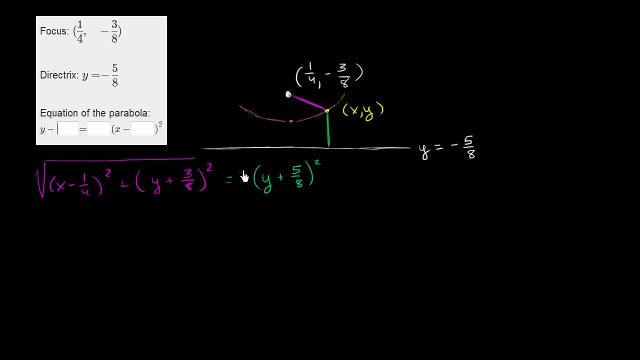 And just to make sure that this is always positive, let's square it and then take the square root. Now, to simplify this, we could square both sides of this equation And we get x minus 1, fourth squared, plus y, And actually let me expand this out. 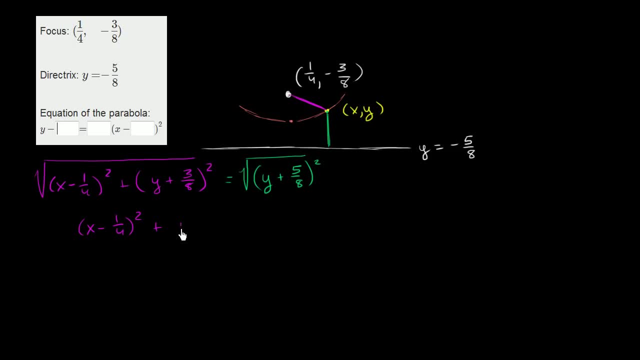 This will be useful for us in a second, So let me expand this out. So this is going to be y squared plus, let's see, 2 times 3 eighths is 3 fourths. So plus 3 fourths, y plus 9 over 64 is equal to this thing. 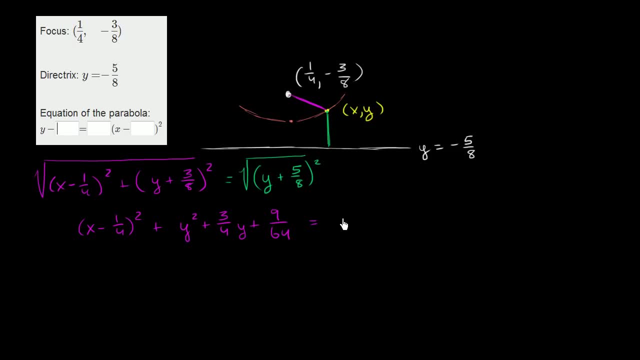 squared, which is just y. Well, let me actually expand that out as well. So that's y squared plus 2 times 5. eighths is going to be 5 fourths, y plus 25 over 64.. Now let me see if I can simplify it. 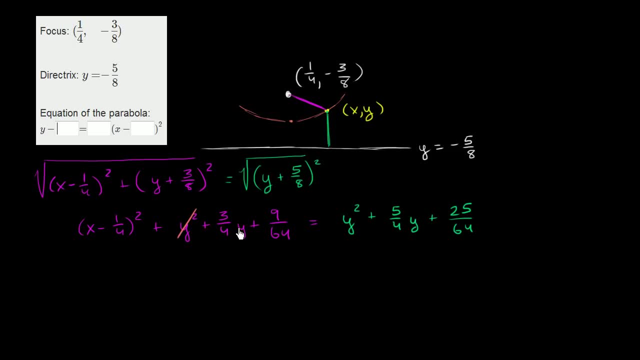 I have a y squared on both sides, So I can cancel those terms out. So y squared, y squared. Let me subtract 3 fourths y from both sides. So let me subtract 3 fourths y. Subtract 3 fourths y. 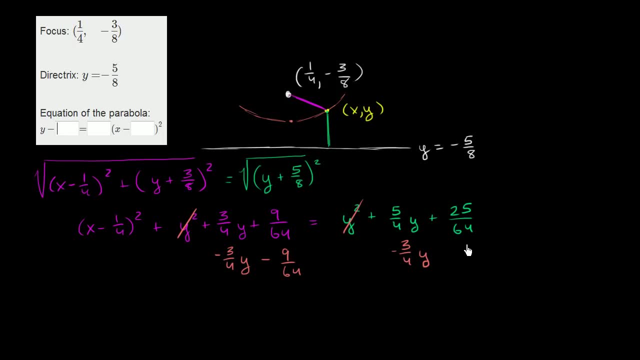 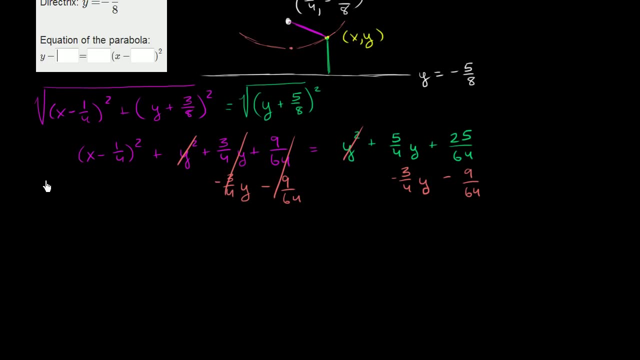 And let me subtract 9: 60 fourths from both sides, Minus 9: 60 fourths, minus 9: 60 fourths. Make sure we have a little more space. So that's going to be gone. That's going to be gone. 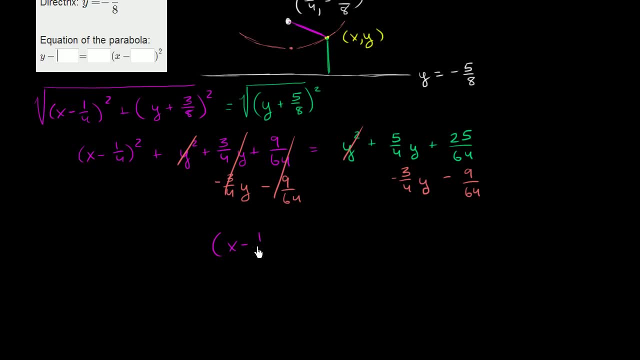 Our left-hand side is just going to simplify to: x minus 1 fourth squared And that's going to be equal to- let's see: 5 fourths minus 3 fourths is 2 fourths, which is the same thing as 1 half y. 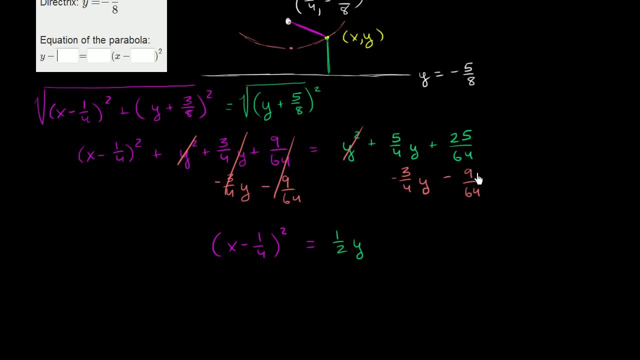 And then 25: 60 fourths minus 9: 60 fourths is 16: 60 fourths, which is just the same thing as 1 fourth. So it's going to be plus 1 fourth there. Now We're almost got where we need to go. 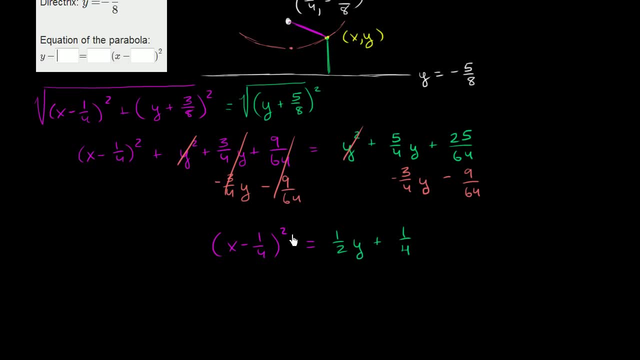 We have this x minus 1, fourth squared. We just need to get a coefficient out here and write this in terms of y minus something. So what we can do right over here is we can factor out a 1 half. So let's do that. 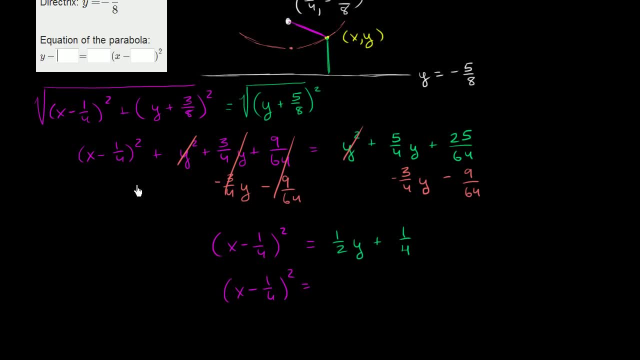 So this is going to be x minus 1. fourth squared is equal to factoring out a 1 half. it's 1 half times y plus 1 half. And now, in order to put it in the form that they care about, 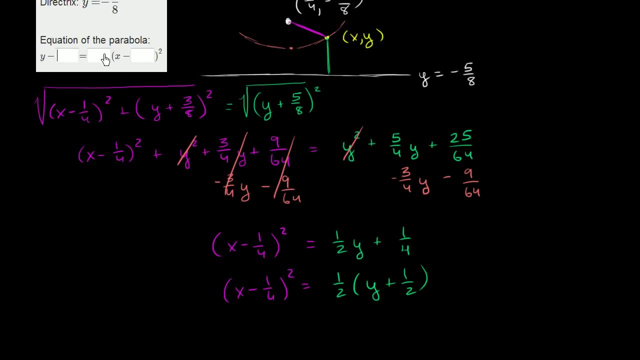 they just have y minus something Right over here, And then something times x minus something squared. So we need to get this 1 half or get this coefficient on the other side. The easiest way I know how to do that is to multiply both sides. 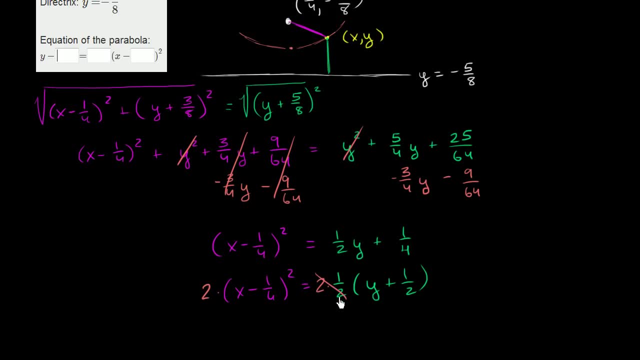 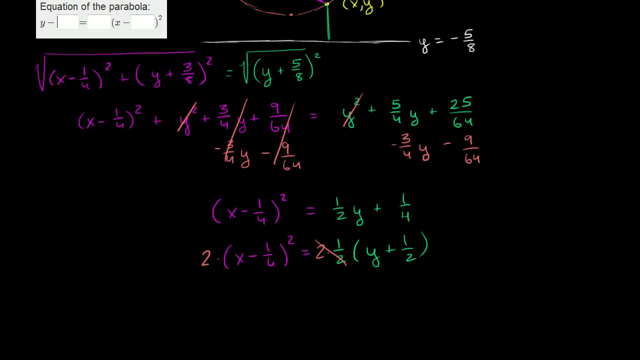 by 2. So you multiply both sides by 2. That cancels And we're left with- and if we really want to put it in the form that they care about, we can swap the sides Instead of writing y plus 1 half. 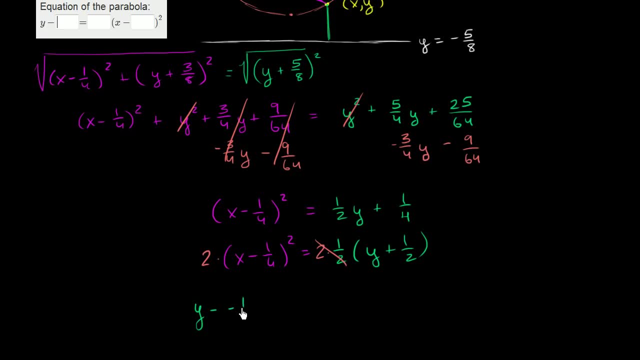 we can write that as y minus negative 1 half. That's the same thing as y plus 1 half. I'm going to do it in the same form that they want Is equal to 2 times x minus 1, fourth squared. 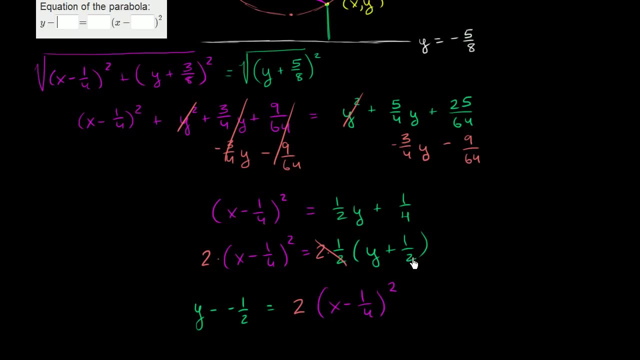 So let me see, Did I do that right? Yep, y minus negative 1 half the same thing as y plus 1 half is equal to 2 times x minus 1, fourth squared. So let me see if we got that actually right. 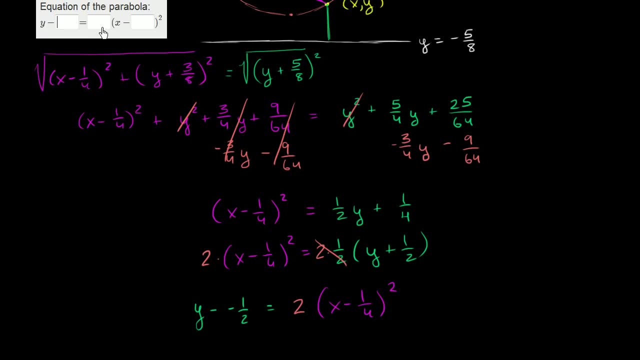 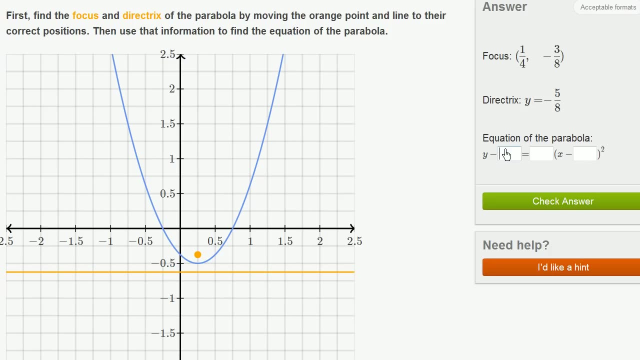 So let's see: y minus, It's negative 1 half, So we have 1 half here, positive 2, and then 1 fourth. So we have: it is negative 1 half, positive 2, and then 1 fourth. 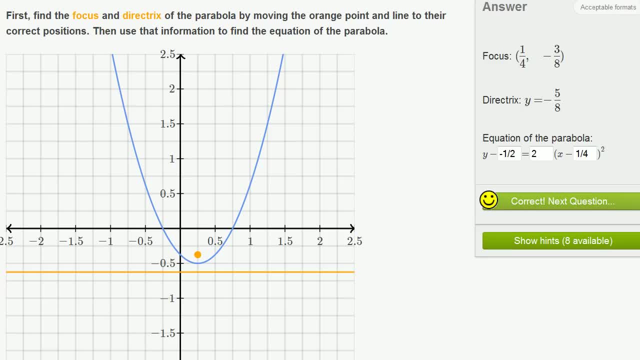 1 over 4.. Let's see if we got it right And we did. 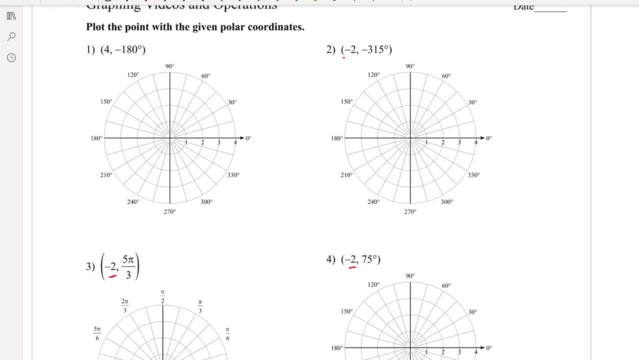 Okay, this is how this works. Notice, mostly we have been having a positive radius and a positive theta And I always say: find the theta first, then go out that far of the radius. You're kind of doing the same thing. You always find the radius first, So negative 180.. So we're